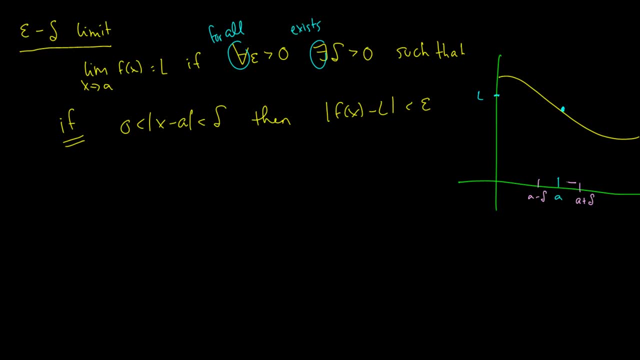 and the same distance here is a minus delta, so this distance here and this distance here is the same. then if this is our range of our point a, then we know that the limit is going to be between two points: l minus epsilon and l plus epsilon. 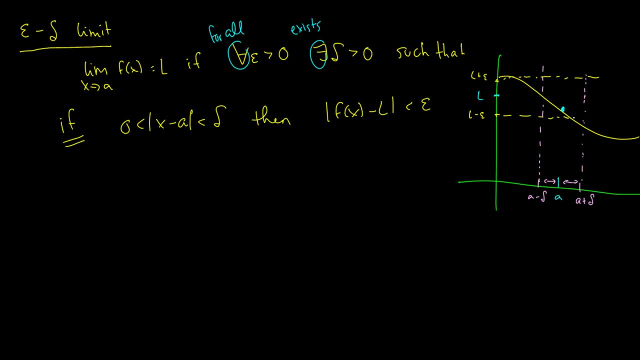 So essentially what it's saying is that if a is somewhere in this distance, then the limit is somewhere in this distance here, And it kind of makes sense. You kind of understand what's going on. It's going to be somewhere in this box. 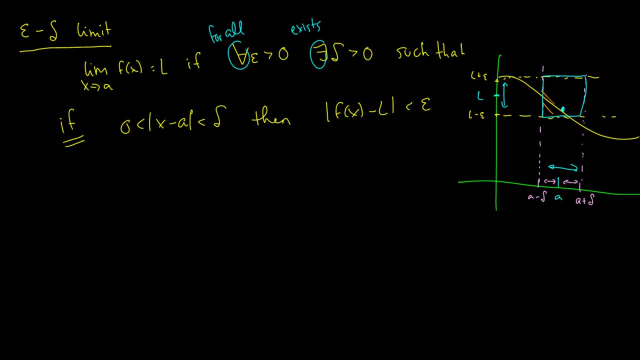 You don't exactly know where, but as long as it's there, then the limit exists. If it's not there, then the limit doesn't exist, And I think that that should make good enough sense for the example coming up. Okay, so you're going to use this? 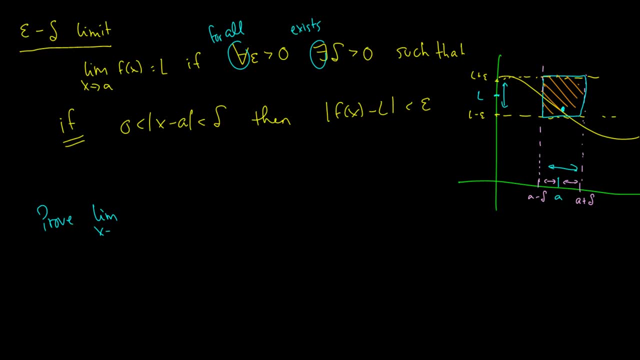 to prove that the limit as x approaches 3 of- let's take 4x minus 5, is equal to 7.. And you're saying now: how do I figure out how to take this graph and this definition and prove a limit, when I could easily just plug 3 into x there? 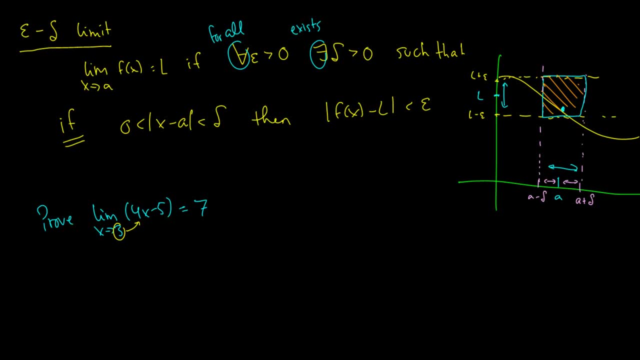 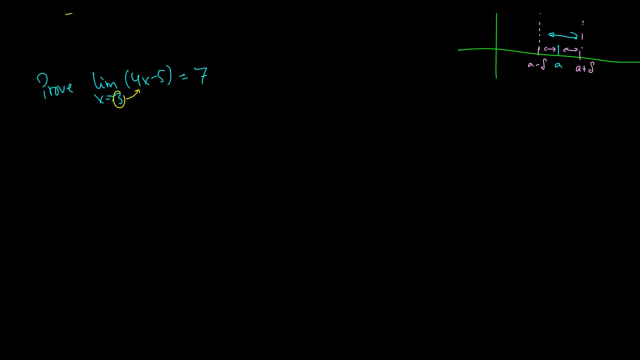 and solve it and it'd be done. Well, this is what I'm here for, because this example can be very challenging. So we're going to start out by filling in the spots in our definition. So we know that if 0 is less than x minus a, 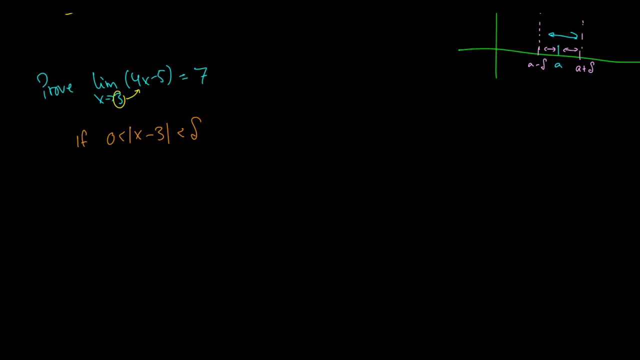 which happens to be 3, is less than some number delta. then our function 4x minus 5, minus our limit, 7, is less than some number epsilon. Okay, so what we're going to do is we're going to work with this number here. 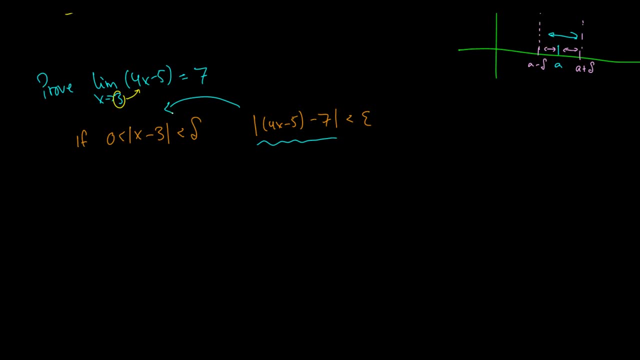 to get it equal to that there, because we are going to guess a delta. So we're guessing a delta And if we guess a delta then we can pick that delta and we can see if we can get it out to become an epsilon later. 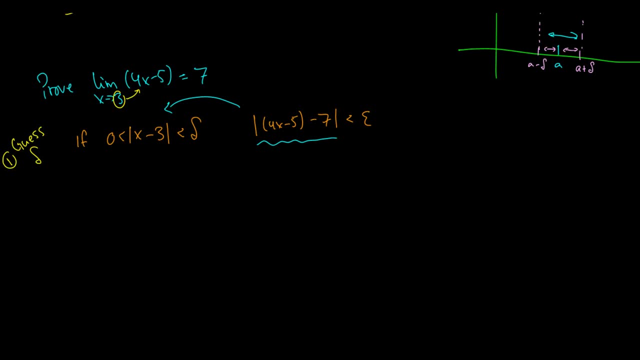 And if it does, then we know that the limit exists and we have our proof. Okay, so this also means that 4x minus 12 is less than epsilon. We can factor out: a 4x minus 3 is less than epsilon. 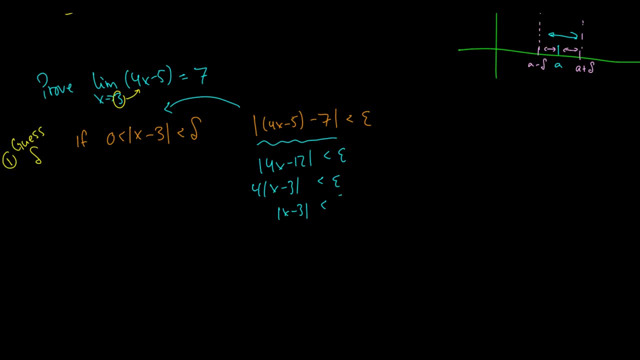 and we can divide by 4.. So this is less than epsilon over 4.. So now we know that the absolute value of x minus 3 is less than delta, And the absolute value of x minus 3 is less than epsilon over 4.. 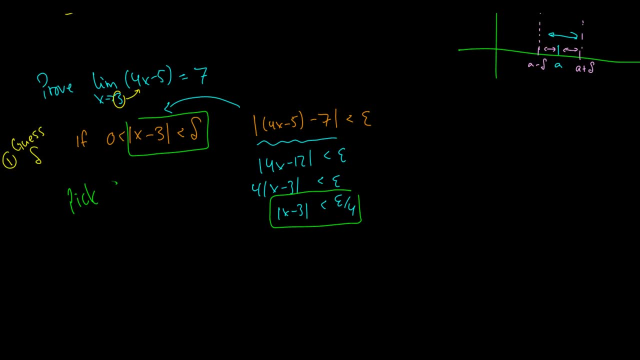 So what we're going to do is we're going to pick delta equal to epsilon over 4.. Okay, so that is one half of the problem. Second half, once you have your delta, is very simple. Now we're going to make sure it works. 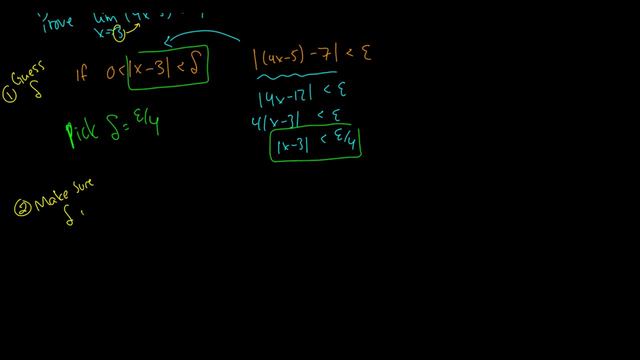 So make sure delta works. Okay, so we're going to start with the right side again. So we're going to say: 4x minus 12 is equal to 4 times x minus 3.. And what do we know about x minus 3?? 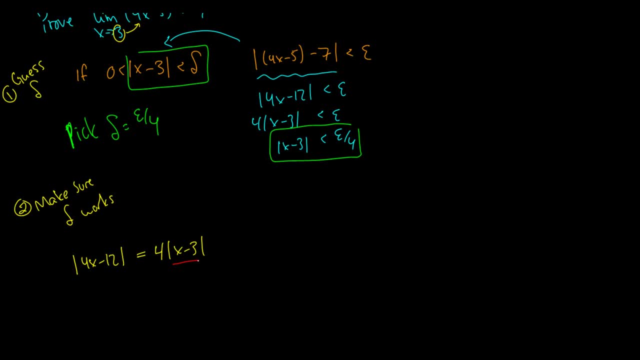 We know that x minus 3 is less than or equal to, actually not less than or equal to. just x minus 3 is less than delta. Okay, so x minus 3 is less than delta. So what we'll do is then we know that it's less than 4 times delta. 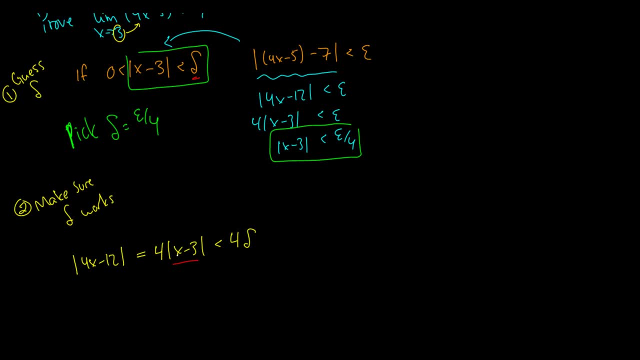 because if x minus 3 is less than delta, then 4 times x minus 3 is less than 4 times delta. But what did we pick delta to be? We picked it to be epsilon over 4.. So this is equal to 4 times epsilon over 4,. 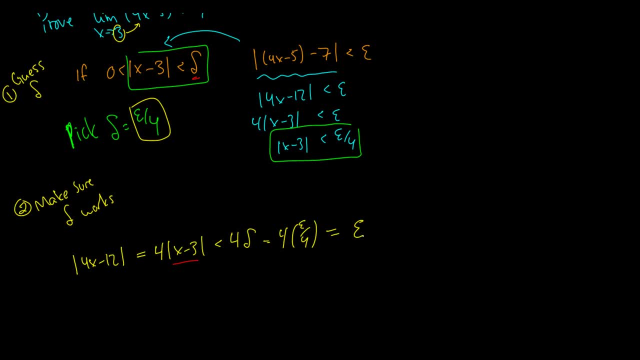 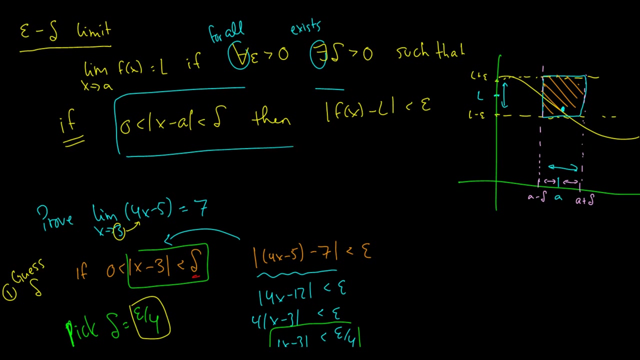 which is equal to epsilon. So we know it worked, because by picking delta equals epsilon over 4, we got epsilon out of it. So now, because of that, we have proven that this statement is true, because we picked a delta here. 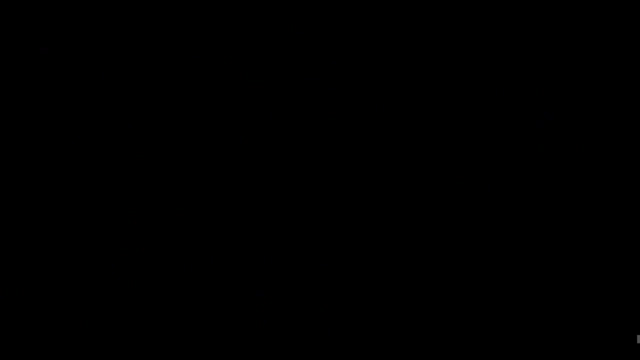 and we got an epsilon out there. So because we picked those two numbers and it came out to be true, thus the proof is complete. So proof complete And that would be a full 6 out of 6 marks on your question. 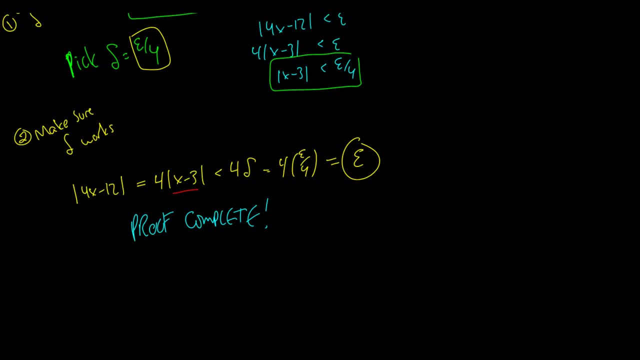 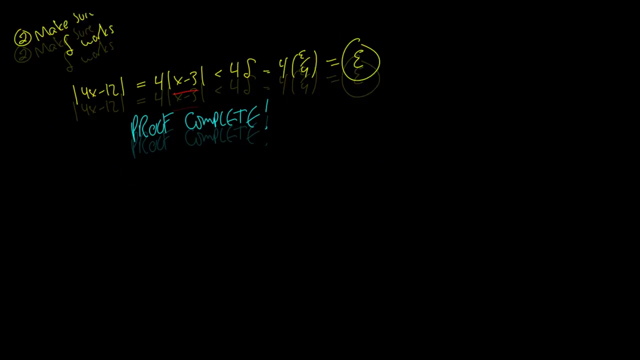 if you had it. So I'm going to give you guys one more question before I leave. let me find a good one here and we'll try it together. All right, let us try. I like this one. This one might be a little bit tricky. 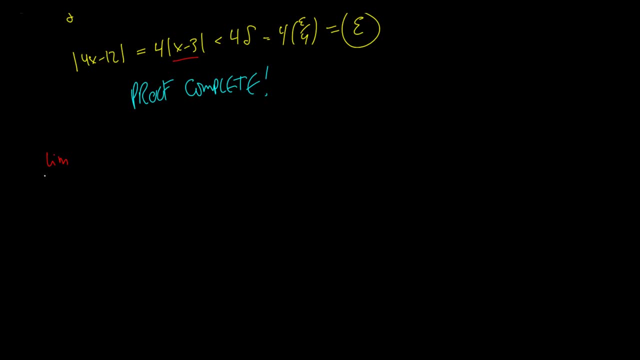 Okay, so here's your question: Prove that the limit, as x approaches 1, of 2 plus 4x divided by 3 is equal to 2.. All right, so pause the video. take some time to do it and I'll show you how to do it when we come back. 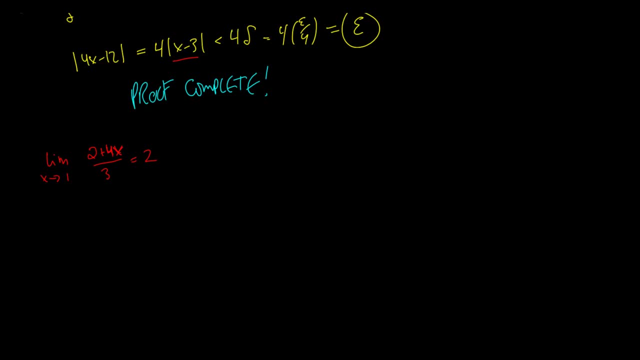 All right, let's tackle this problem. So let's set it up. We know that x minus a is greater than 0, which is x minus 1, which is less than our number delta, and we know that our function minus our limit is less than the number epsilon. 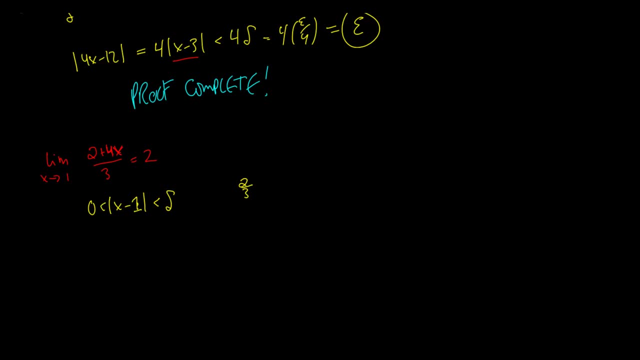 So we have- I'm going to break this into fractions- 2 thirds plus 4 thirds x minus 2, which I am actually going to make this into fractions. so I'm going to make 6 thirds, just to make it easier for you guys to see what's going on algebraically. 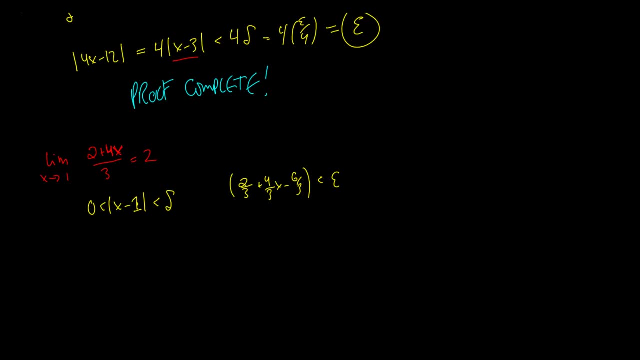 is less than epsilon. Okay, so if we want to somehow make that that, Okay, so let's subtract So negative: 4 thirds plus 4 thirds x is less than epsilon. Of course these are absolute values. So if we just take out 4 thirds, 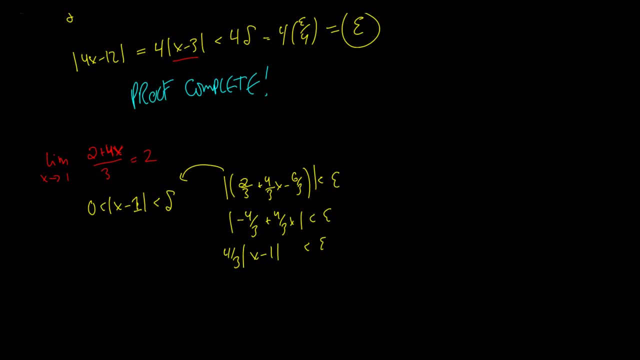 then that's: x minus 1 is less than epsilon. So we know that x minus 1, is going to be less than we're going to divide by 4 thirds on both sides. So that is 3 epsilon over 4,. 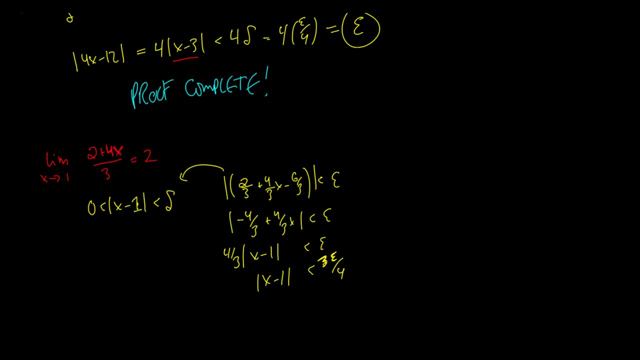 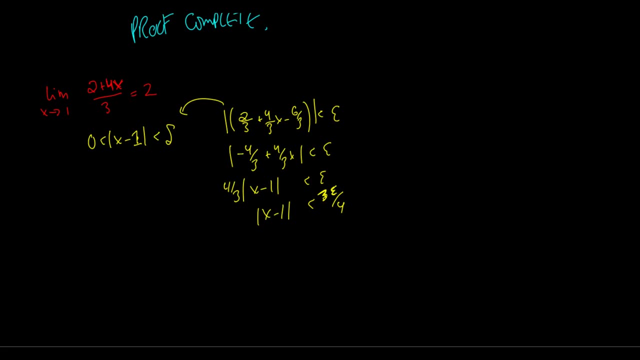 and my threes and epsilons look very similar. So I'm terribly sorry for this example. I'll try to do something about that now. So we've gone one direction, We've done step one, We've picked a delta and we're going to pick. delta is equal to 3 epsilon over 4.. 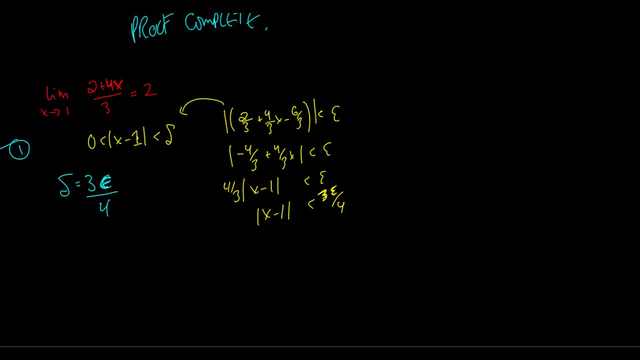 I'll use this epsilon. It's used in set notation, but it'll do better for differentiating my writing in this example. Okay, so now in step two, we want to start with the same thing we started with before. So we know that the absolute value of